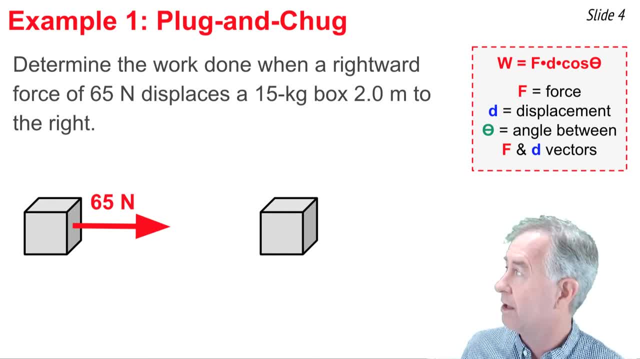 So I begin with a diagram. I show the initial position of the box, the final position of the box and the force acting upon the box is 65 Newtons. It acts over a displacement value of 2 meters. I want to know the angle between the force and displacement vector. 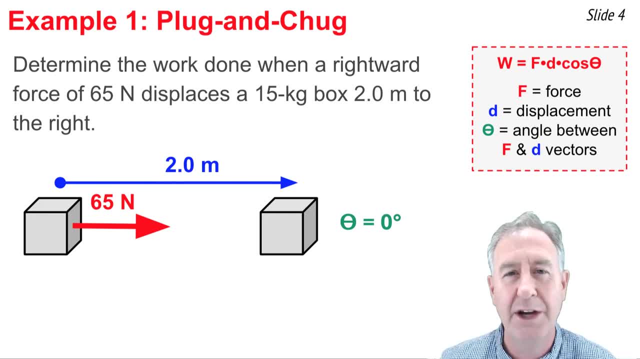 When they go in the same direction. that angle is 0 degrees. Now I take my value of force and my value of displacement and I substitute it into the equation for work. I put 0 degrees for theta and the cosine of 0 is 1.. Using my calculators, the value 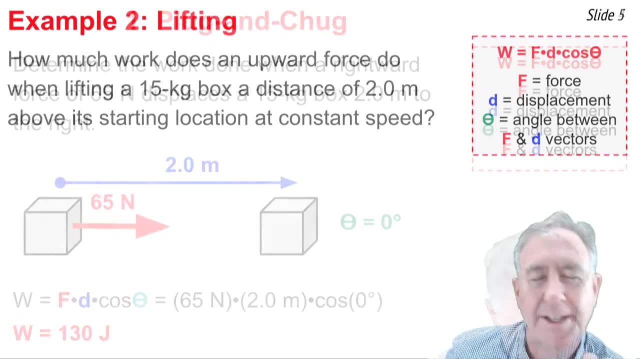 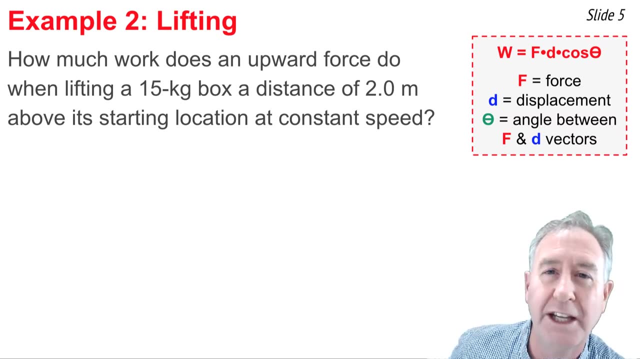 of work is 130 joules. The second example involves a lifting motion. I want to know how much work does an upward force do when lifting a 15 kg box a distance of 2 meters above its starting location at a constant speed? Once more, I need to know the force, the displacement and the angle. 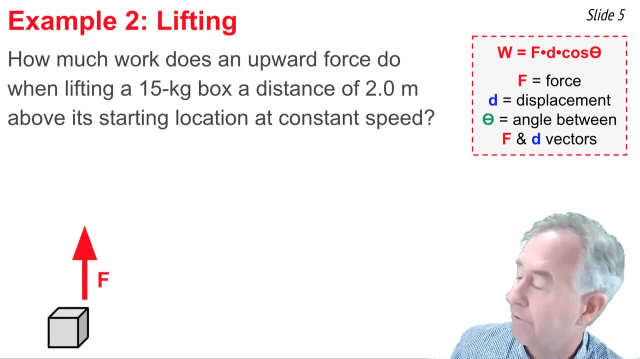 between force and displacement. So I begin with a diagram and I have the initial position of the box with a force acting upward on it to move it to its final position, two meters above its starting location. So I know the value of D but I'm not given the value. 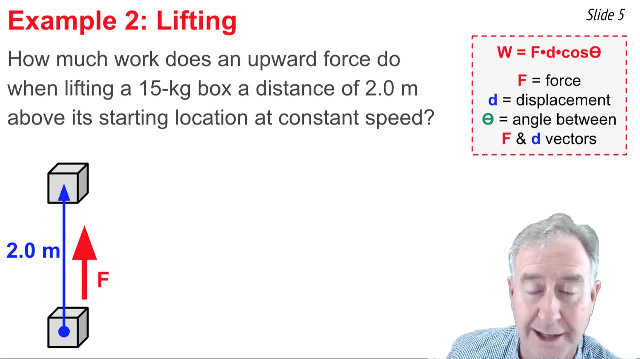 of F, But what I know is that the box moves at constant speed in a straight line, which tells me that the forces must balance, which means the upward force that I'm trying to determine must be equivalent to the downward force of gravity, Knowing that the force of 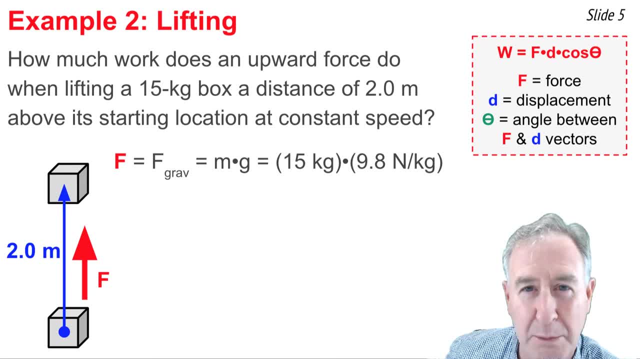 gravity is equal to m times g. I can calculate this upward force. The mass here is 15 kilograms. I multiply it by 9.8 newtons per kilogram and I get an upward force of 147 newtons. I now know F and D and the angle. theta is simply the angle between these two vectors. 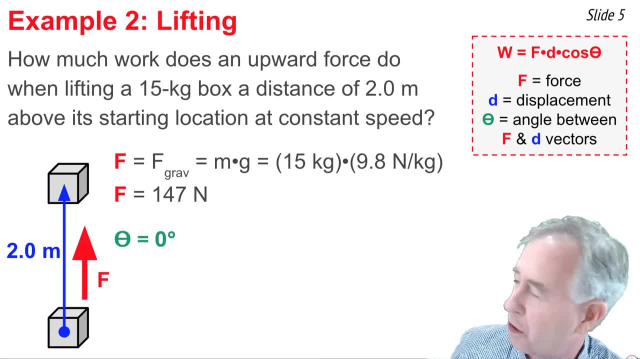 the force vector and the displacement vector When they go in the same direction. that angle is zero degrees. Now I'm ready to use my work equation. I take 147 newtons, I multiply it by 2 meters and I multiply it by the cosine of the angle between F and D. The cosine of zero is one. 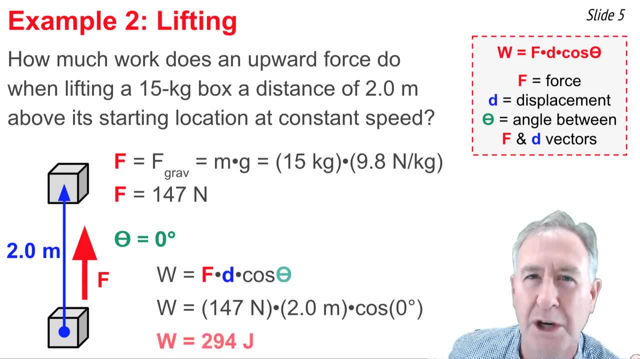 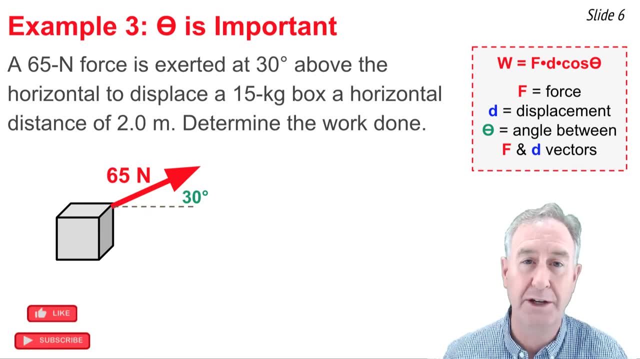 and so 147 times 2 gives me a work value of 294 joules. In our third example we want to know the work done when a 65 newton force, exerted at 30 degrees above the horizontal, displaces a 15 kilogram box a distance of 2 meters to. 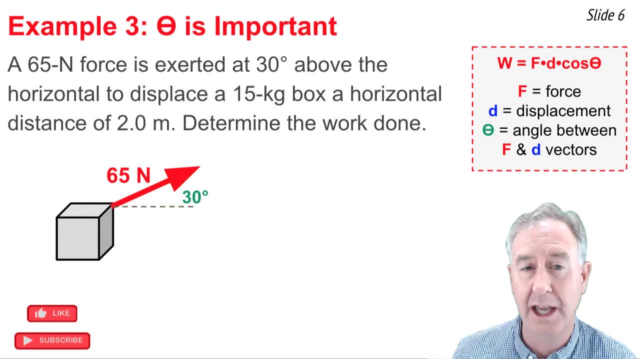 the right. In our diagram we see this force acting on the box and it displaces the box 2 meters to the right. We show that in the diagram. We want to know the angle between the F and the D, Since the D is to the right and the force is 30 degrees above the right the angle. 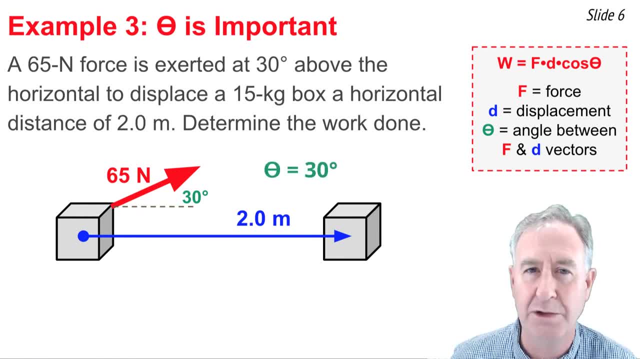 between F and D is 30 degrees. Now I can take my values of F, D and theta and substitute it into the work equation. I go 65 newtons times 2 meters times the cosine of 30 degrees. Using my calculator, I find: 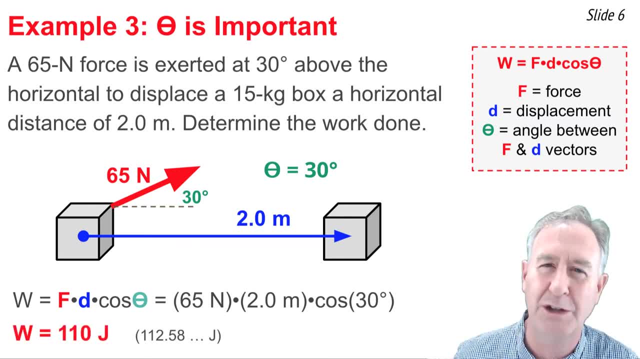 out. the value for work is 1.3.. The work equation is 15 newtons per kilogram. I multiply it by 2 meters and I get a work approximately 113 joules. Now, if I wish to round this to two significant digits, 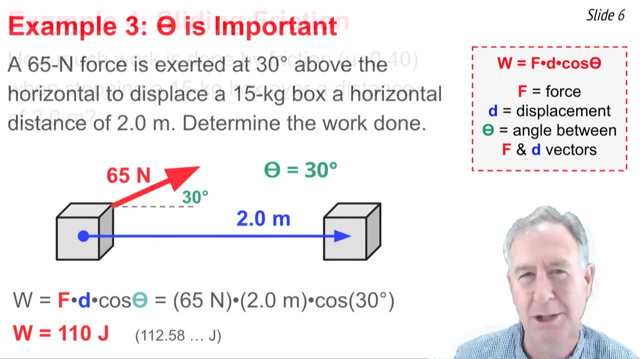 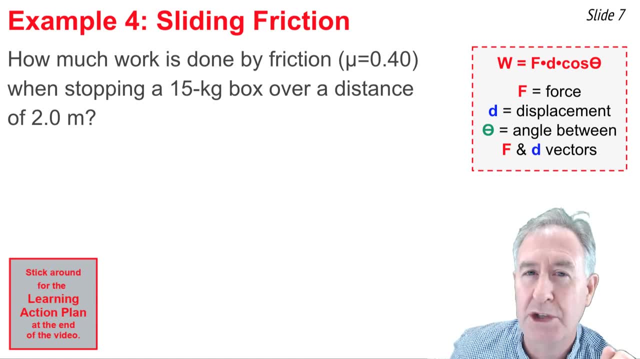 which would be important to some people. then I end up with 110 joules. The fourth example involves sliding friction, and I want to know how much work is done by friction when stopping a 15 kilogram box as it slides to a stop over a distance. 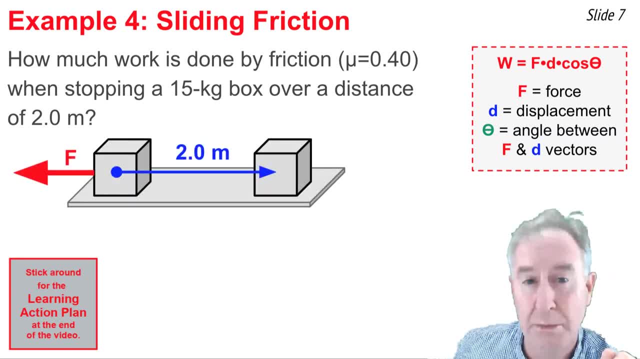 of two meters. So I begin with a diagram and I show the displacement of two meters to the right. Friction acts opposite the box. It's directed to the left, So the angle between the F and the D vector here is 180 degrees typically. 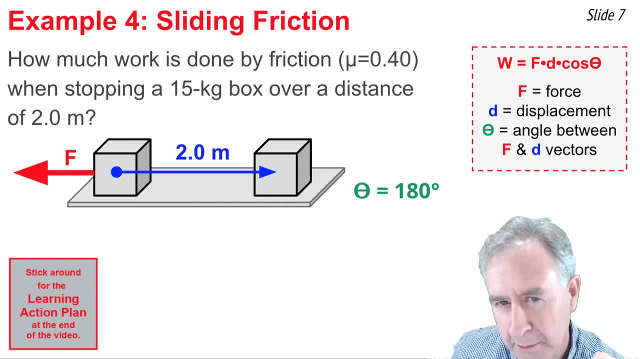 the case for sliding friction forces. Now the crux of this problem involves finding the value for the force of friction. The force of friction is equal to mu times F norm, and for a box on a horizontal surface, F norm is equal to the weight of the box, M times G. So to calculate the force of friction, I go mu. 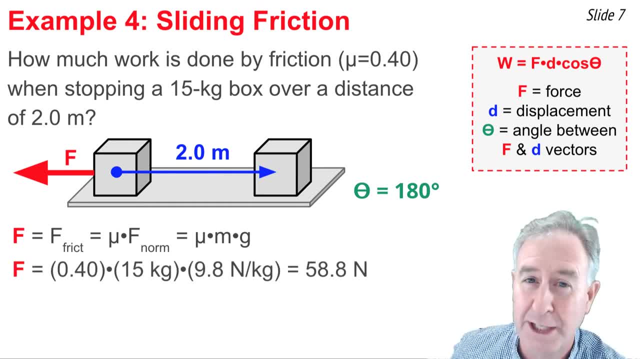 times M times G, That is 0.4 times 15 times 9.8 and I get 58.8 Newtons as the force of friction acting on the box. Now I know F, D and theta and I can substitute it into my work equation: The cosine of 180 degrees. 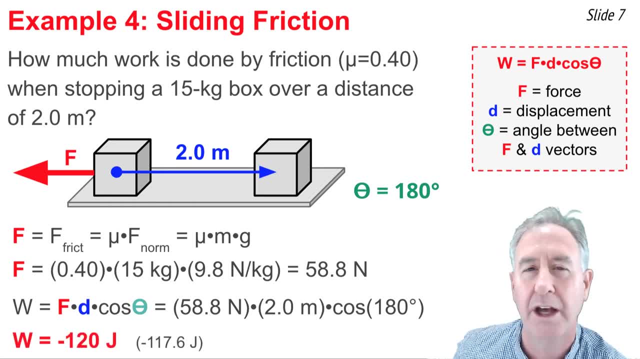 is negative 1 and when I do my math I end up getting a value of negative 117.6 joules for the work done on the box. I can round this to two significant digits, such that the work is negative 120 joules. Our fifth example involves 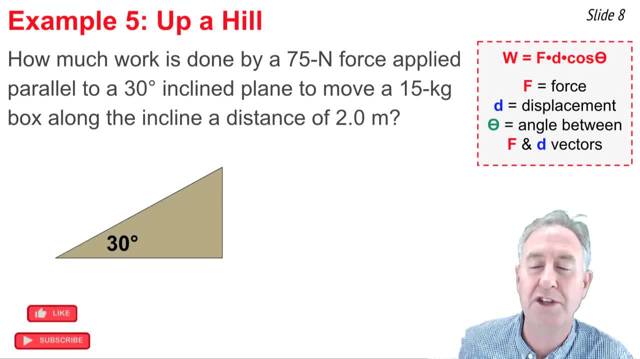 the motion along an incline plane. I want to know how much work is done by the 75 Newton force applied parallel to the incline to move a 15 kilogram box a distance of 2 meters along the incline. So here's my incline plane with a 30. 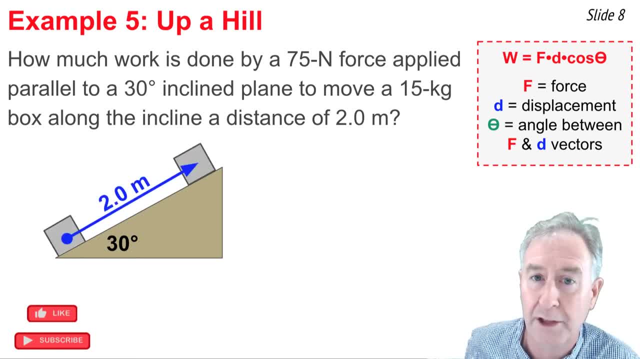 degree incline angle. A box moves along it parallel to the incline a distance of 2 meters because of a force that acts parallel to the incline. I know the F, I know the D and I need to know the theta. Theta is not 30 degrees, That's the. 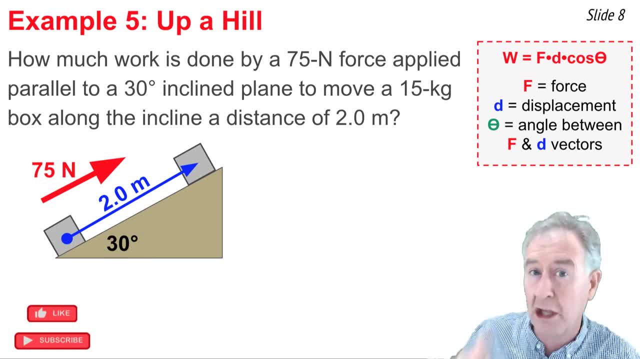 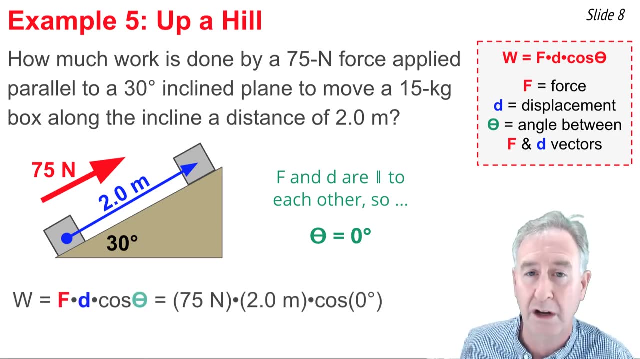 incline angle. Theta in the work equation is the angle between the force and displacement vectors and since they go in the same direction the angle theta is 0 degrees. Now I know F, D and theta. I can substitute into my work equation and I can solve the value of work 75 times 2. 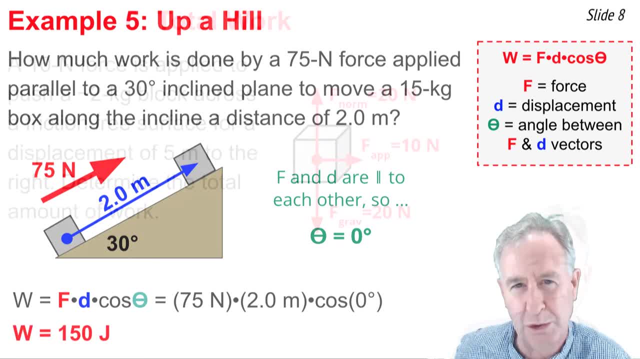 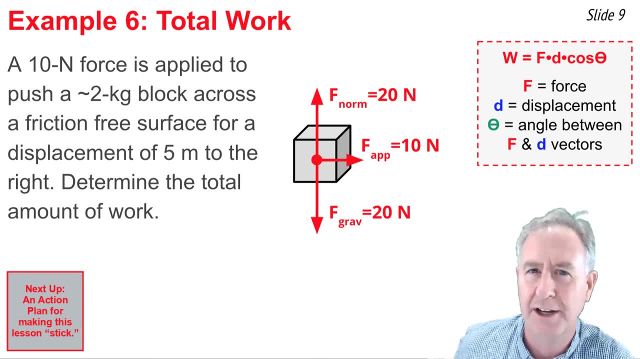 times the cosine of 0 is 150 joules. In our last example I want to determine the total work done when there are multiple forces acting up on an object. A 10 Newton force is applied to push a 2 kilogram box to the right for a displacement of 5 meters across a friction-free surface. 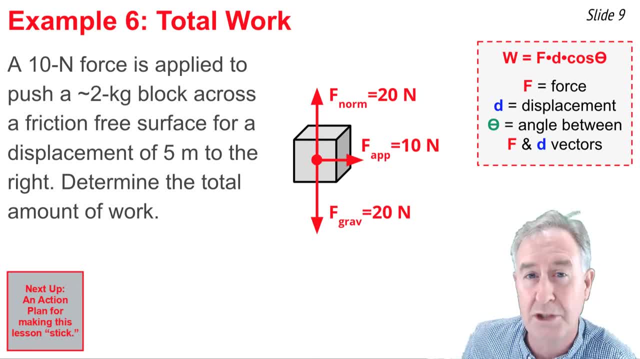 determine the total work done. The free body diagram shows the individual forces, their values and their direction. This object is displaced to the right for 5 meters. In order to calculate the total work done, I need to calculate the work done by each individual force. I'll begin with the two vertical forces For F graph. 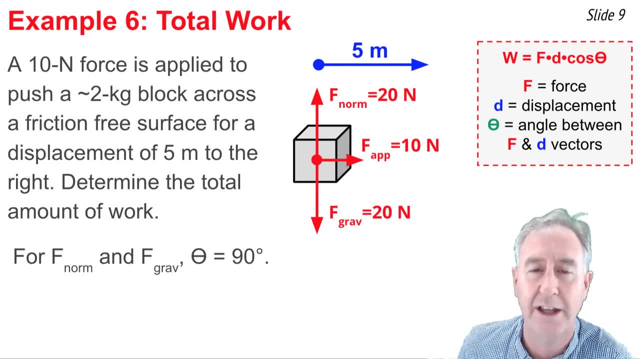 and F norm. the angle between the up and the right and the down in the right is 90 degrees. The cosine of 90 degrees is zero, so the work done by these two forces would be zero joules. Put another way, vertical forces do not do work on horizontally. 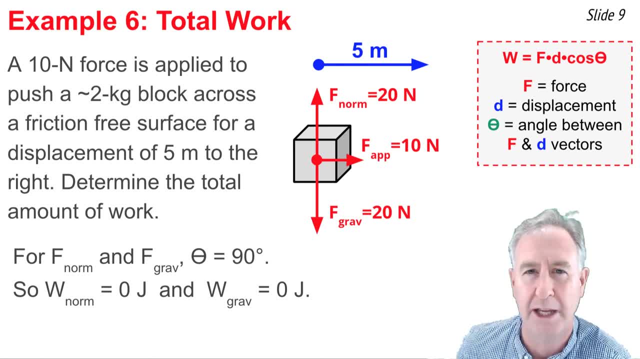 moving objects. That leaves one individual force remaining the applied force. It's directed to the right and the displacement is to the right. so the angle between the applied force and the displacement is 0 degrees. I can calculate the work done by this applied force. I substitute 10 Newtons for F 5.